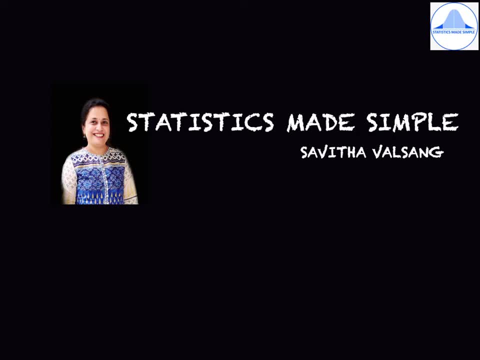 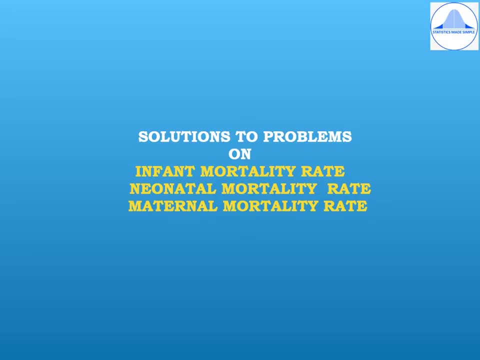 I am Savita Valsang and welcome to my channel. Statistics Made Simple. In this video, we will find solutions to problems based on infant mortality rate, neonatal mortality rate and maternal mortality rate. These problems are usually asked for two marks in the exam, where one mark is allotted for the formula and the other mark is for the calculations and for the final answer. 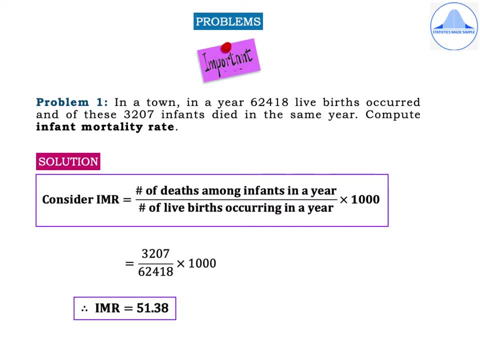 Problem 1. In a town in a year, 62,418 live births occurred, and of them, 3,206 were born. 7 infants died in the same year. Compute infant mortality rate. For the solution, write the formula for IMR, which is equal to number of deaths among infants in a year divided by number of live births occurring in a year, into thousand. 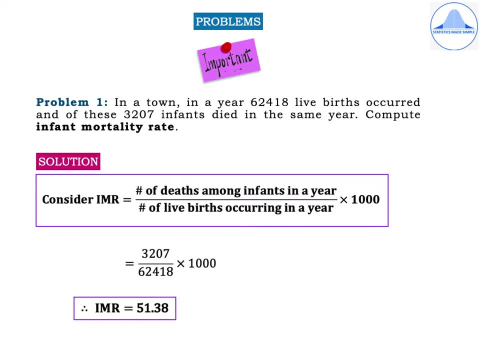 So the formula will carry one mark and next you substitute the values for the numerator and denominator, which is equal to 3,000.. ल. 60,407 divided by 62,418 into 1000.. Therefore, IMR is equal to 51.38. again, here, take only 2 places after the decimal, after rounding off for the final answer. 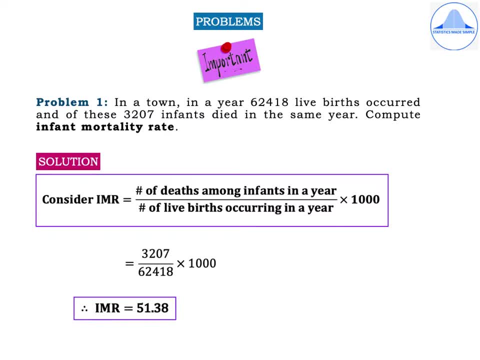 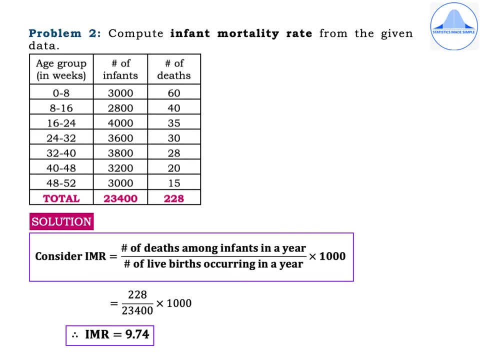 The final Això carries one mark, So totally this is a two mark problem. Problem 2.. 2. Compute infant mortality rate from the given data. In the first column we have age group in weeks: 0 to 8,, 8 to 16,, 16 to 24, 24 to 32,, 32 to 40,, 40 to 48,, 48 to 52. Then 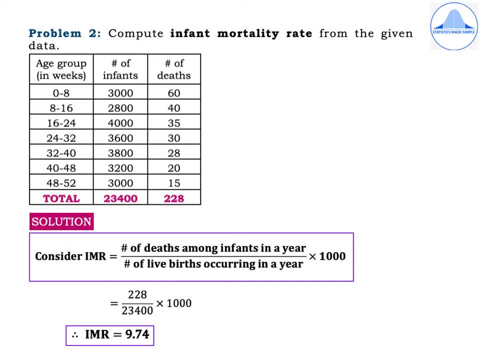 you have number of infants as 3000,, 2800,, 4000,, 3600,, 3800,, 3200,, 3000, and the number of deaths are 60,, 40,, 35,, 30,, 28,, 20 and 15.. Now keep in mind that an infant is a child. 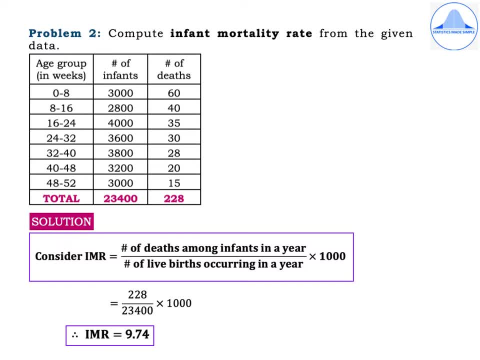 who is aged less than 1 year. So in a year there will be 52 weeks. So that's why in the first column we have age group in weeks, given from 0 to 52.. Now to calculate the infant mortality rate. 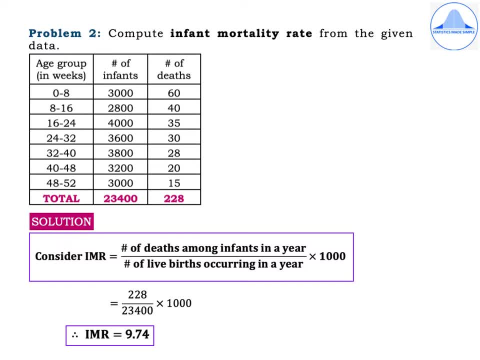 we need the total number of infants and the total number of deaths. So, starting with the solution, write the formula: consider: IMR is equal to number of deaths among infants in a year, divided by number of live births occurring in a year into 1000.. So in the table, 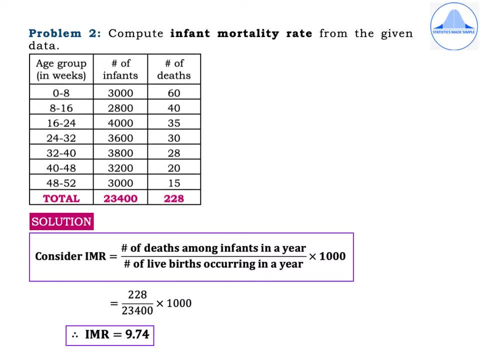 I have formed an extra row in pink color. that is the total, and found out the number of infants, which is nothing of live births, which is 23,400, and number of deaths is 228.. Substituting these totals in the IMR formula, we get 228 divided by 23,400 into 1000.. Therefore, IMR is equal to 9.74.. 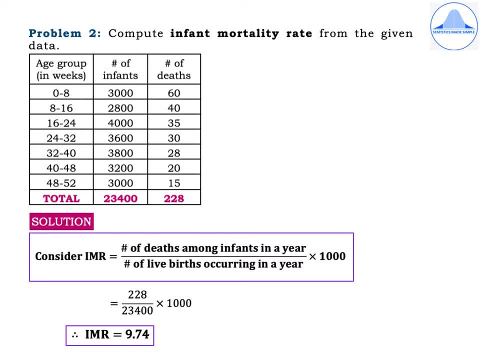 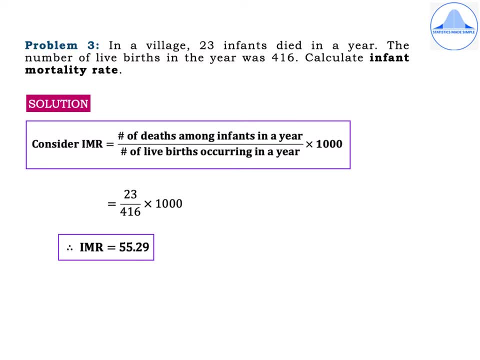 Problem 3. In a village 23 infants died in a year. The number of live births in the year was 416.. Calculate infant mortality rate. Solution. Write the formula. Consider: IMR is equal to number of deaths among infants in a year divided by number of live births occurring. 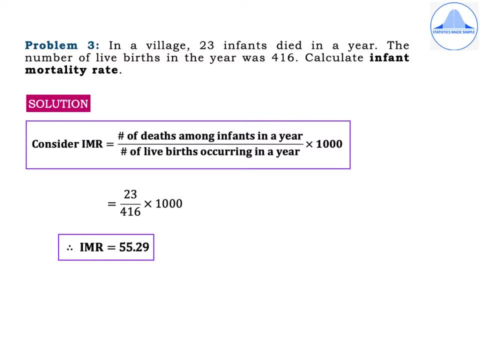 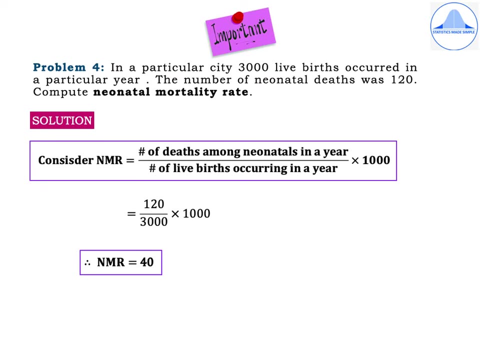 in a year into 1000, which is equal to 9.74.. The number of live births in a village is equal to 23. divided by 416 into 1000, which gives IMR is equal to 55.29.. Problem 4. In a particular city, 3000 live births occurred in a particular year. The 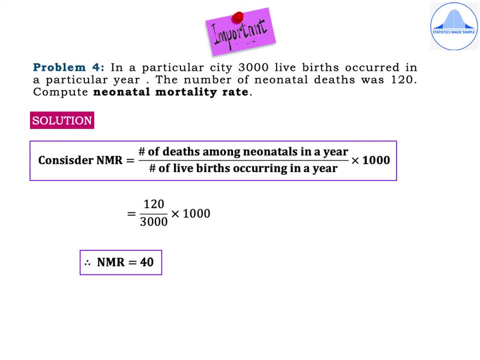 number of neonatal deaths was 120.. Compute neonatal mortality rate Solution. Write the formula for NMR: NMR is equal to number of deaths among neonatals in a year, divided by number of live births occurring in a year into 1000, which is equal to 120 divided by 3000 into 1000.. Therefore, 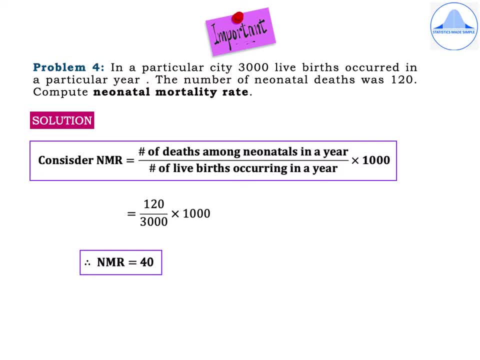 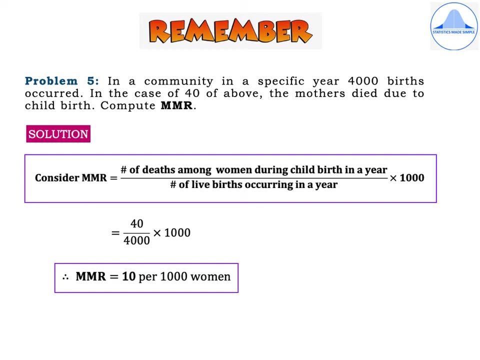 NMR is equal to 40.. Recollect that a neonatal is a child under 28 days of age. Problem 5.. In a village, 23 infants died in a year. The number of neonatals in a year is equal to 25.. In a community, in a specific year, 4000 births occurred. In the case of 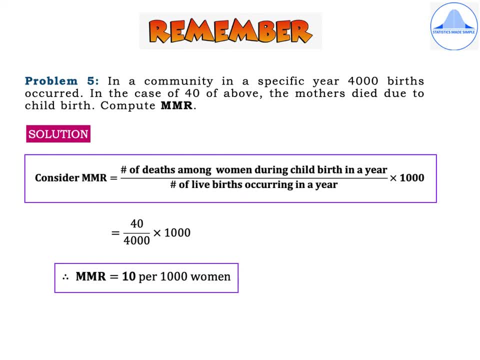 40 of the above, the mothers died due to childbirth. Compute MMR, So MMR stands for the maternal mortality rate. Start with the solution. Write the formula for MMR, which is equal to number of deaths among women during childbirth in a year, divided by number of live births occurring. in a year into 1000, which is equal to 9.74.. The number of deaths among women during childbirth in a year, divided by number of live births occurring in a year into 1000, which is equal to 40 divided by 4000 into 1000.. Therefore, MMR is equal to 10 per 1000 women. 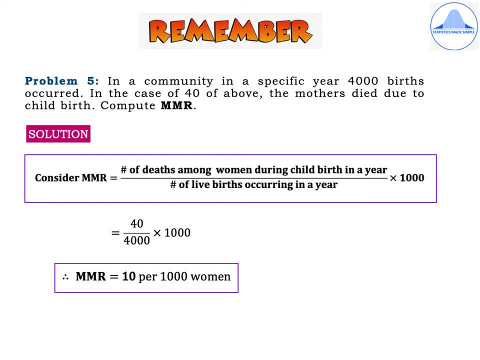 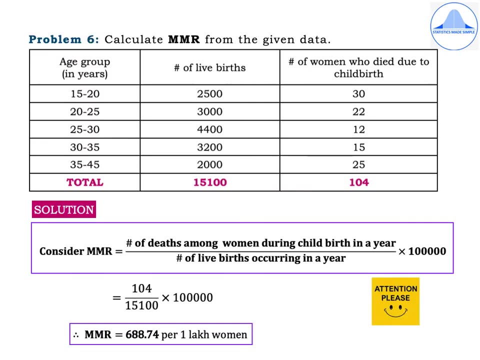 MMR formula can be expressed either in terms of 1000 or 1 rack. This particular problem: we have expressed MMR in terms of 1000.. Problem 6. Calculate MMR from the given data. We have age group in years: 15 to 20, 20 to 25,, 25 to 30,, 30 to 35,, 35 to 45. And the 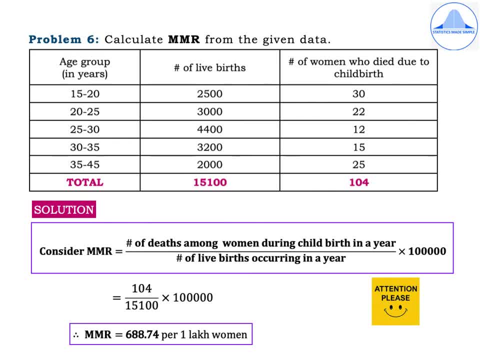 number of live births are 2500, 3000,, 4400, 3200, 2000.. And the number of women who died due to childbirth are 30, 22,, 12,, 15 and 25.. Now, starting with the solution, Write MMR. 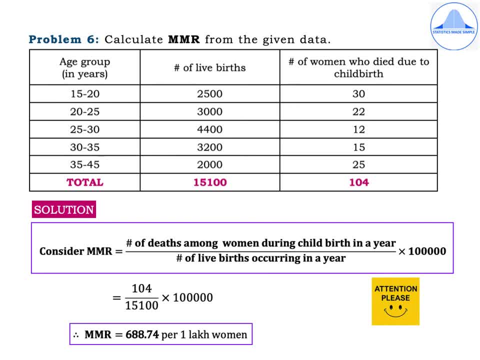 formula, MMR formula- which is equal to number of deaths among women during childbirth in a year divided by number of live births occurring in a year, into 1 rack. So here I have expressed the MMR formula in terms of 1 rack. In the given table I have found out an extra row that 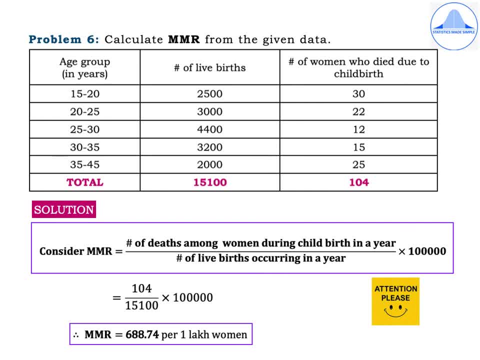 is the total. And the total number of live births are 15,100.. And the number of women who died due to childbirth is 100.. And the total number of live births are 15,100.. And the total number of live births are 15,100.. And the number of women who died due to childbirth.